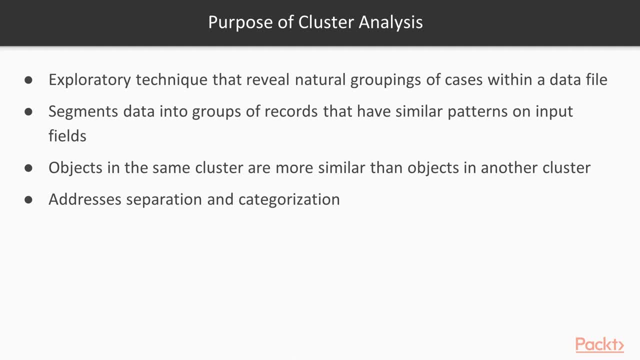 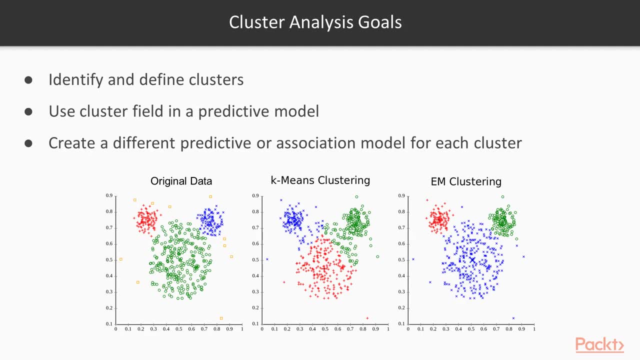 Or the same types of customers. Instead, we have different students or customers, or whatever it happens to be, that have these different patterns within the data. Now, the goals of cluster analysis are really three reasons why you do cluster analysis. The first is really that you 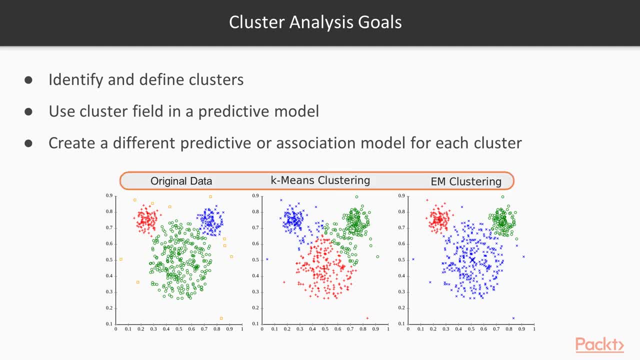 just want to identify and define your clusters. So, again, rather than just treating everybody as being similar, we know that there are these different patterns within our cases, within our data, and we want to identify these different patterns and create these different groups so that we can look at them differently and see how they really behave. A second 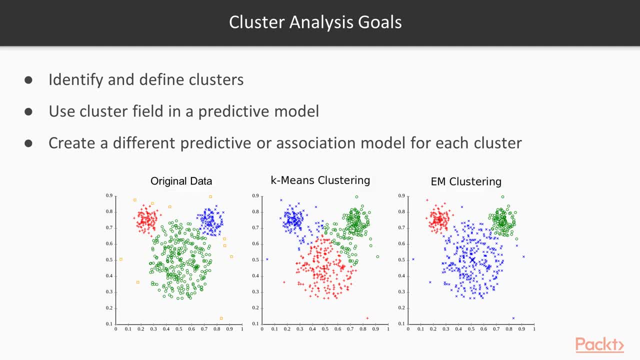 reason why you might do cluster analysis is that cluster analysis may not be the end goal in and of itself. Instead, you might do a cluster analysis. you see these different groups, you identify them, but then you use that cluster field and you use that as another. 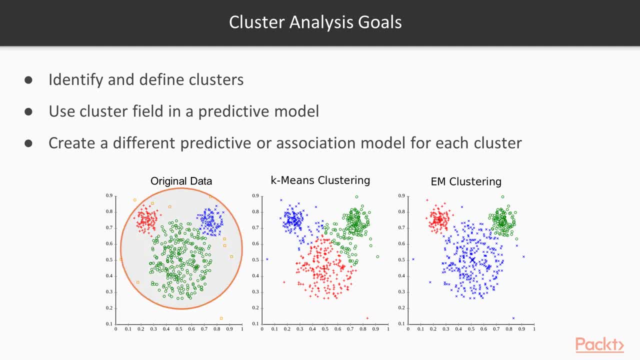 variable in a predictive or associative model. So, again, knowing that extra piece of information is just another variable that you can use to try to improve the predictive models that you're building. A third reason why you might do cluster analysis is that you take the perspective that these clusters or groups, 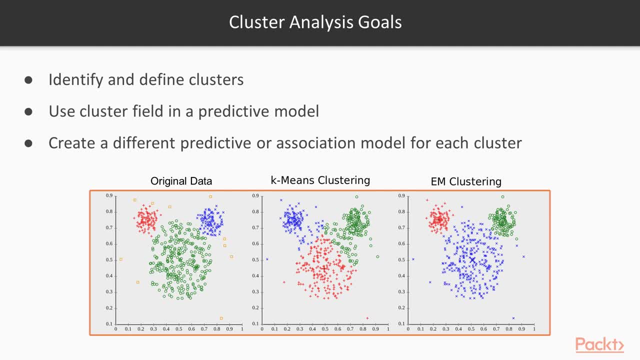 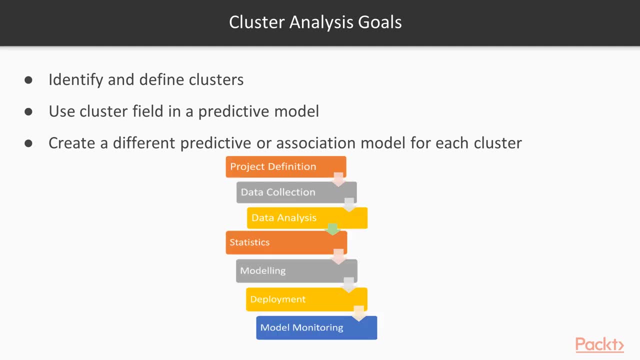 are so different from each other that you really need to separate each group and create different predictive or association models for each cluster. So the idea there is that building one model for the entire data set is not really good enough. Instead, these groups are so. 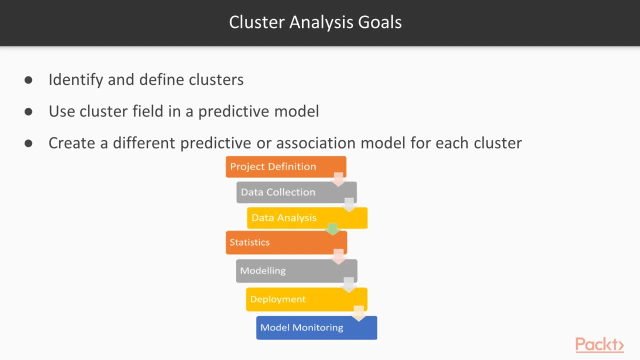 different, that they're going to have different patterns within our variables of interest, that we really need to create separate models for each group, And so you're basically almost using a cluster analysis to figure out how to build a cluster analysis for each cluster. So that's. 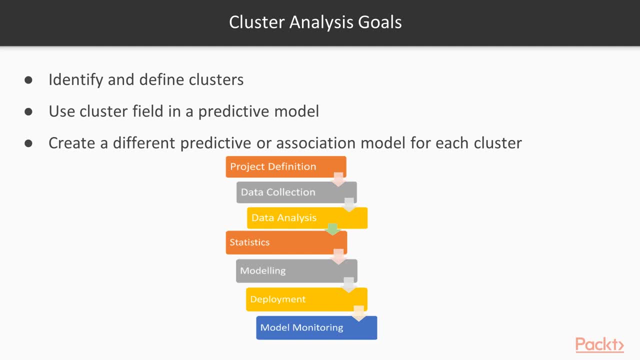 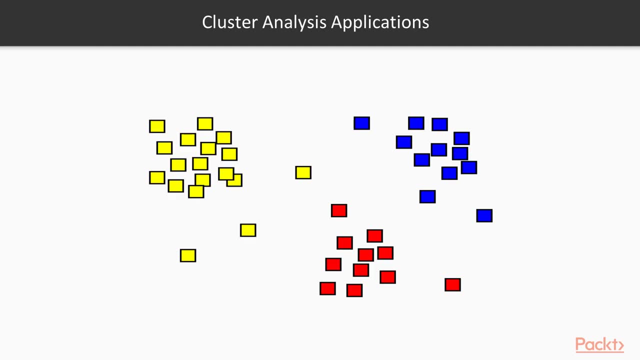 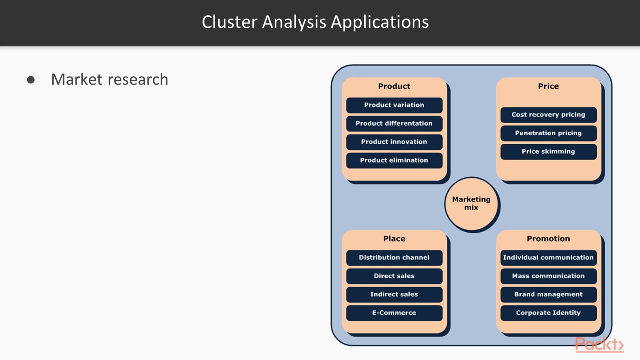 really a way to separate these different groups and create different models for each one of them. Now, in terms of applications for cluster analysis, first and foremost, it's been used in market research, So, for example, we may find that there are different buying patterns for our customers. 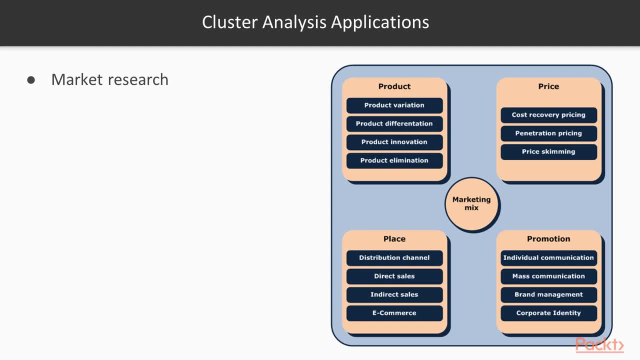 and we may want to create different marketing campaigns for each one of them so that we don't all get the same advertisements, but the advertisements are targeted. As an example, a few years ago I worked on a project where we were doing a project where we were doing a 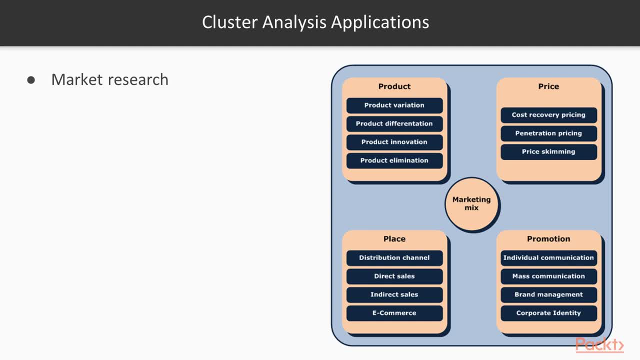 political targeting and, rather than approaching each potential voter with the same piece of information, we targeted the voters so that those voters that were more interested in social issues got information on the social issues of these different candidates and those voters that were more interested in economic issues got information on the financial or economic stances of these. 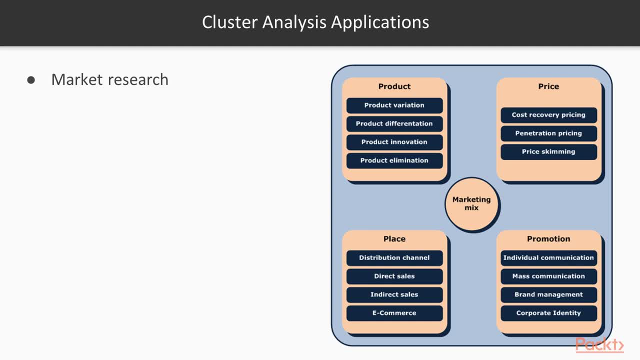 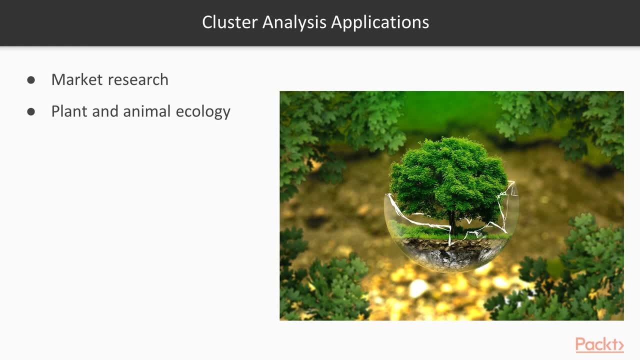 different candidates. So, again, your marketing becomes much more targeted and specific to those people that might be interested in that. Another way you can use cluster analysis is you can use it in plant and animal ecology. So, again, we want to just separate these different plants or animals into different species and genus, and 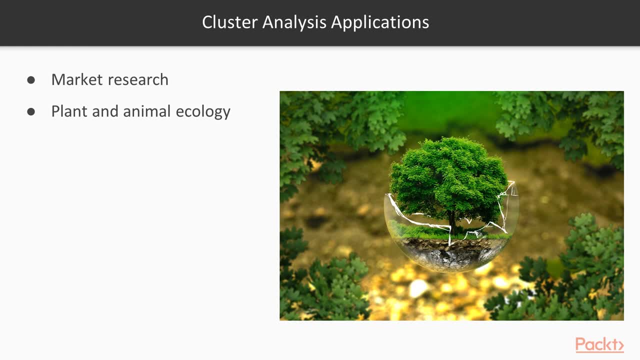 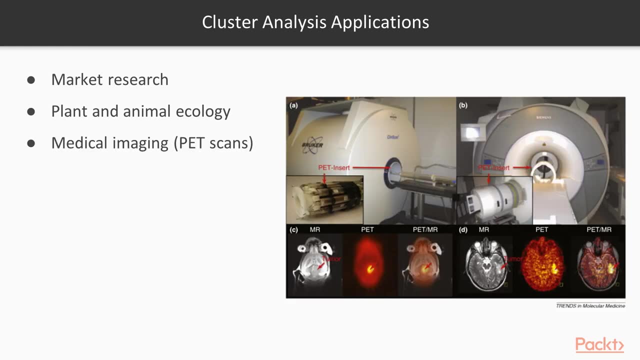 so forth. We can do that by doing cluster analysis, seeing what characteristics certain plants share with each other and things like that, so that we can create these different families. Another example of how we could use cluster analysis is in PET scans, for example. So again, 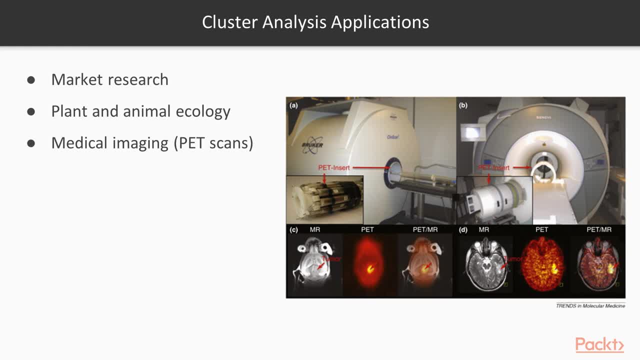 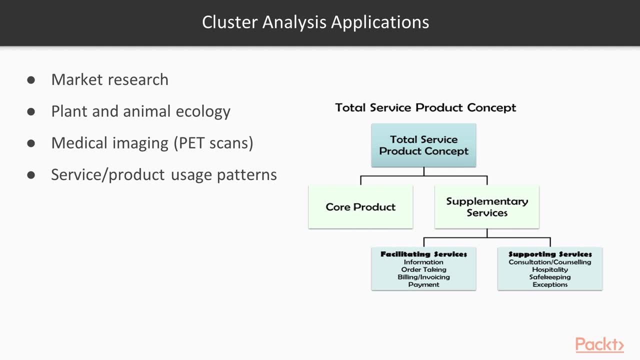 we're seeing these different clusters, maybe in terms of brain activity and things like that. Another area where you could use cluster analysis is we might be looking at service and product usage patterns. So we may have a group of outpatients, for example, and we want 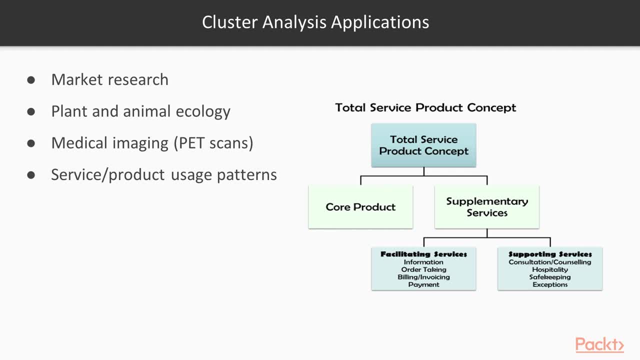 to see what services they use And that way we can see, you know, whether we have some people that are users of all different types of services or maybe they only use some specific services, and things like that. We also can use cluster analysis for social network analysis. We could use it for 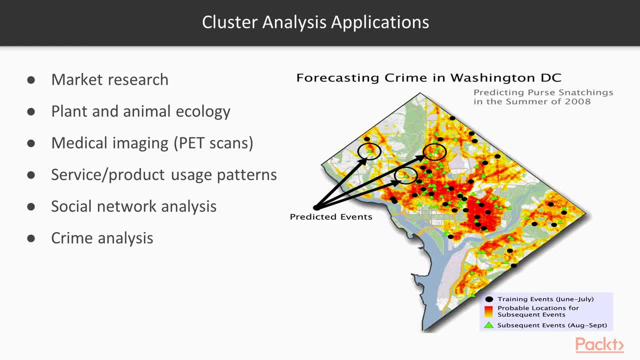 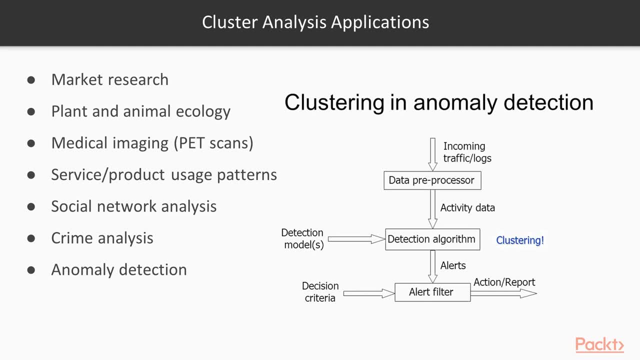 crime analysis to kind of find out where different crimes are taking place within a city and things like that. Or we may want to use cluster analysis for anomaly detection, not only to identify outliers, for example, but we could use it to identify things like cases of fraud or where 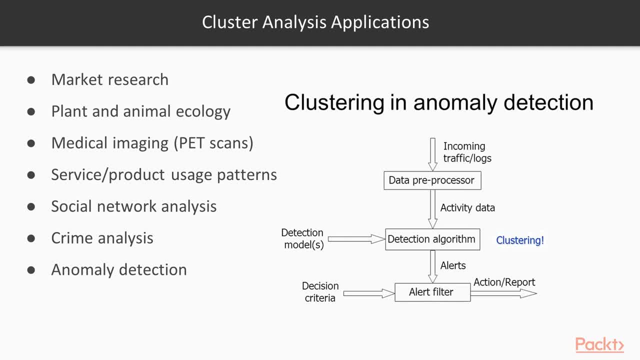 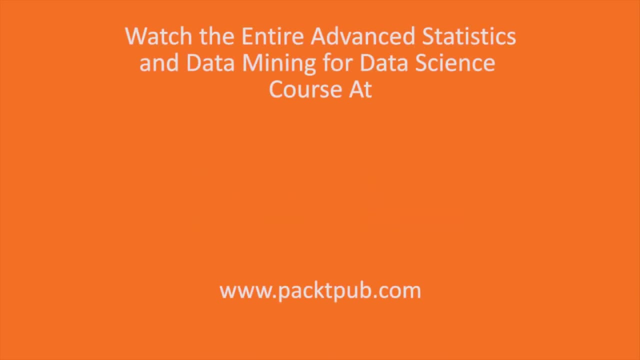 something unusual is happening. For example, a few years ago I worked on a project where we were trying to identify cargo containers that were carrying illegal items. And we didn't manage to identify the cargo containers that were carrying illegal items. So we had to think of how to do the things that we could do, And I think you know we've seen. again: like what? in the case of like, for example, when it comes to like two or three or four truckloads of cargo, you know, you know, you know like, keep it direct. and you know like, if you spend money on your cargo, it's less than a million dollars. So if you were to go, through the thing that you'd do. you know, even if you were to through the term, you could keep it direct, because you're trying to find something that would don't even have any.